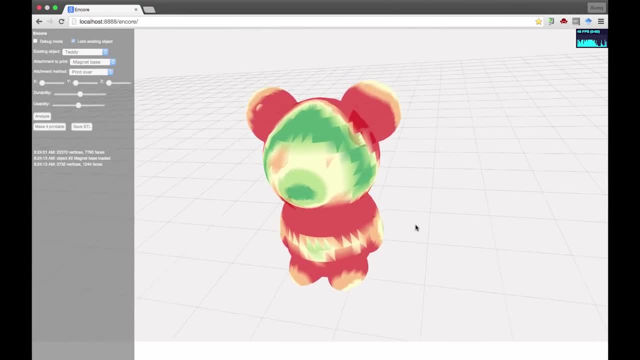 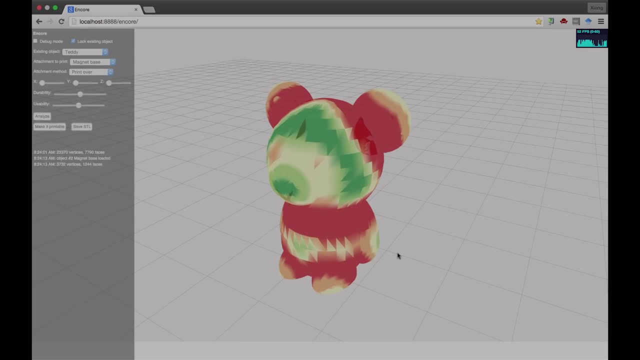 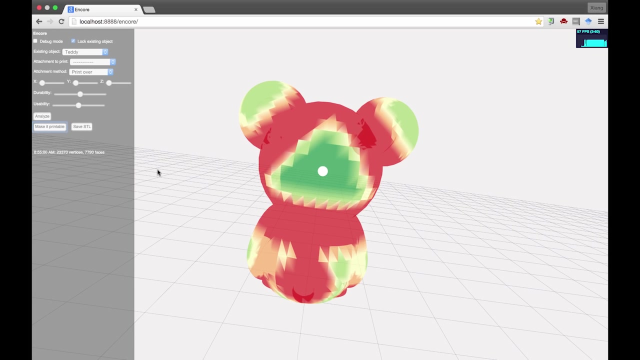 onto the surface of an existing object. Our analysis and visualization highlight areas of the object where printing attachment will cause collision problems. The user simply clicks at the point of interest. The system then orients the object so that the selected area can be reached by the printer. The system then orients the object so that the selected area can be reached by the printer. 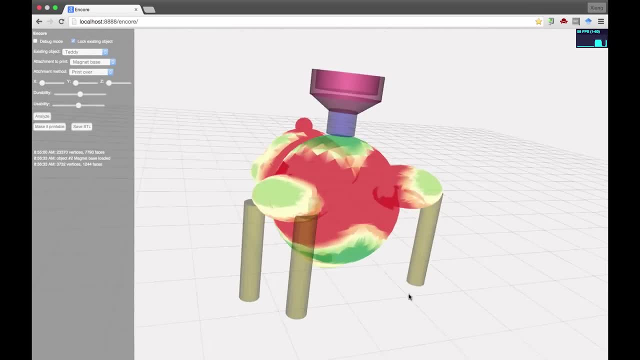 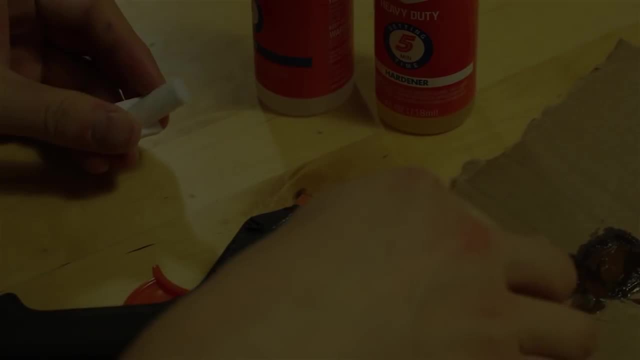 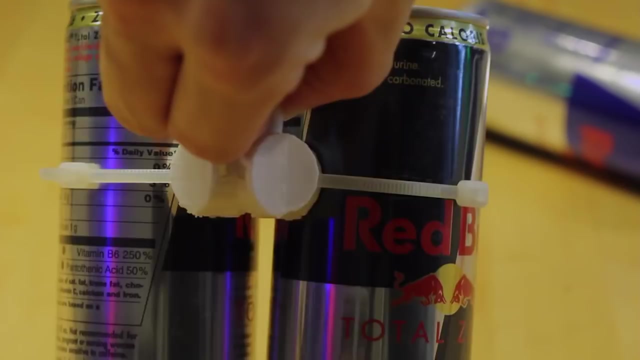 It also creates scaffolding structure that holds the object in place, so that the printer can directly print the attachment on top of it. The second technique, print to affix, generates an attachment that can be affixed to the object using external mechanisms such as adhesives or straps. We use constructive, solid geometry. 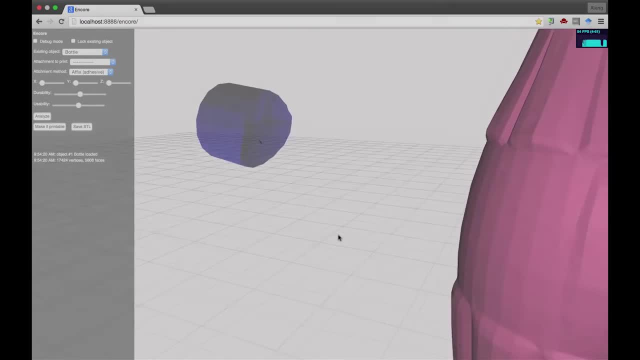 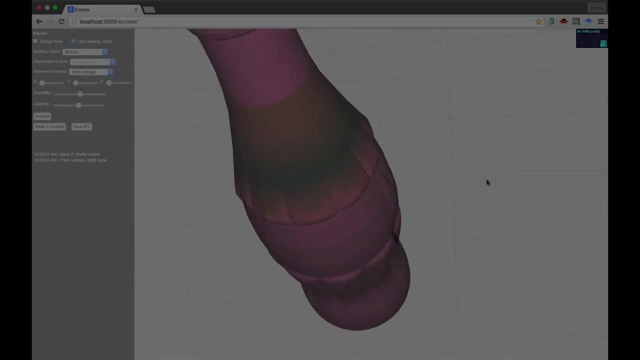 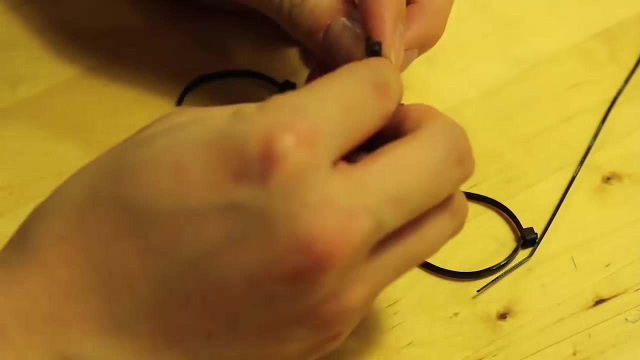 to make the handle snug fit to the area the user selects To use strap. the user simply draws on the object to indicate which way the strap goes. The attachment is then made strappable using zip ties or velcros. Straps also make attachment reusable, such as this simple battery casing. 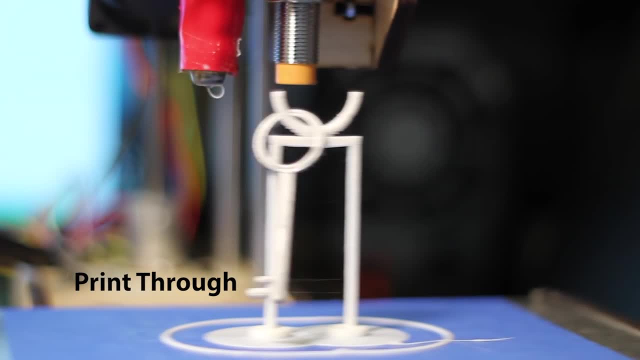 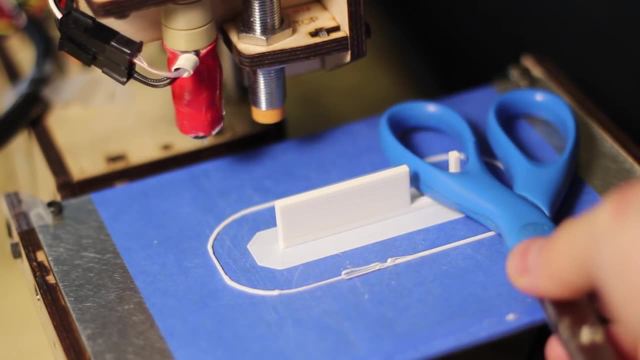 The third technique: print through prints, an attachment through the hole of an existing object. For example, for the scissor name tag, the printer is paused the midway And the scissors are placed onto the print bed so that the name tag goes through one of its handles. 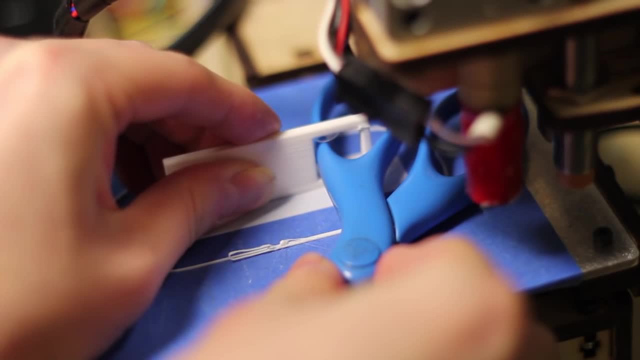 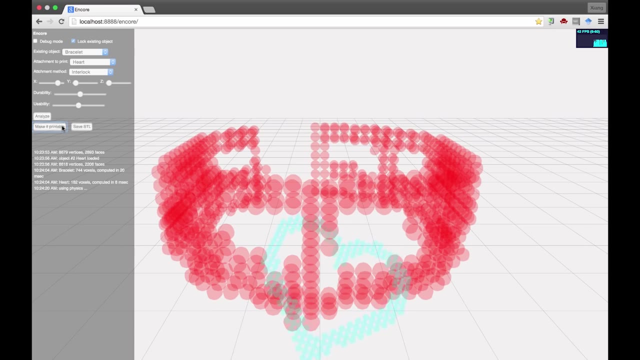 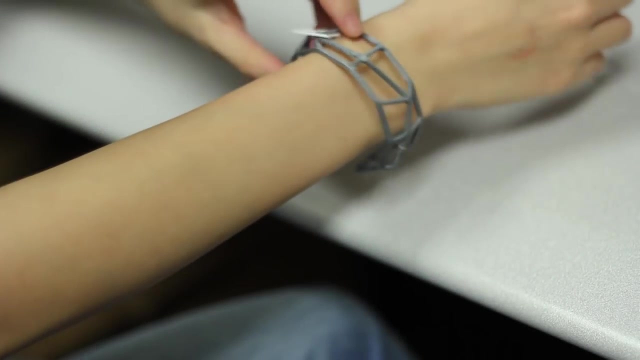 When the name tag is finished printing, it is already attached to the scissors without using any external mechanisms. We perform a physics simulation to tell the user when to pause the print so that the object can be dropped without interfering the printhead. We evaluated these attachment techniques. We also added the 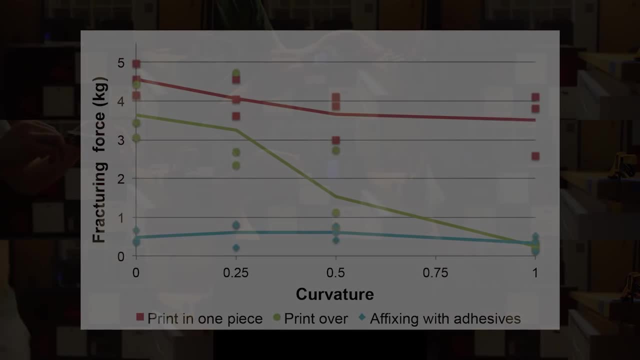 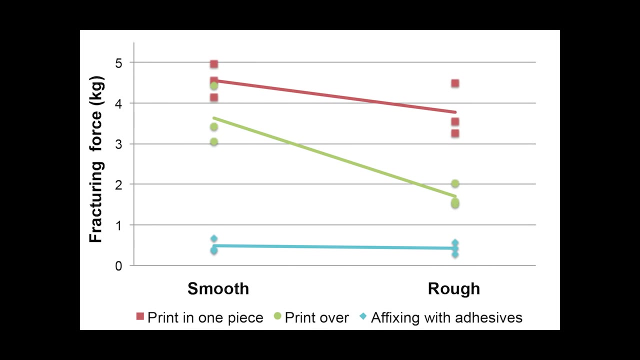 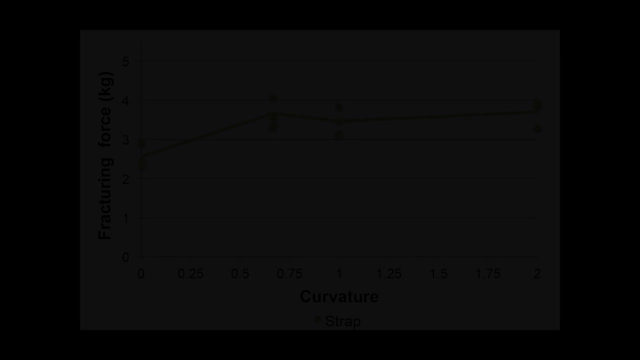 with a stress test. The results show that using adhesives creates a weak attachment. Other techniques overall show promising strength compared to the baseline approach, but all suffer from changes in the surface curvature and roughness. To summarize, we show that 3D printing can be used not just to build objects from scratches. 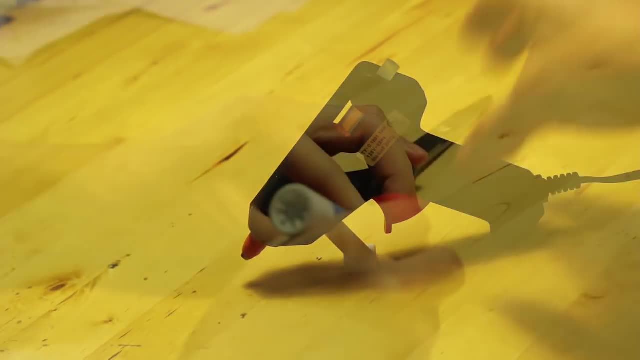 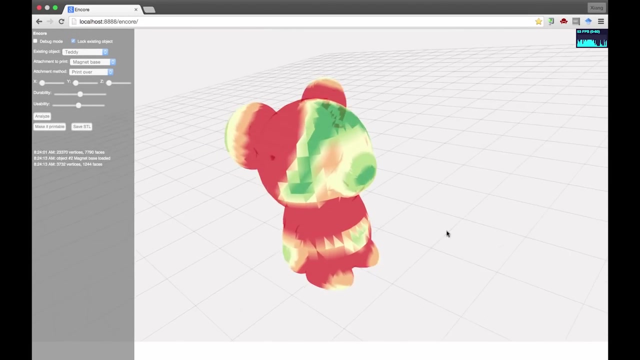 but also to augment objects that already exist in our everyday life. All techniques and computational framework serve as a point of departure for designers, developers and makers to further explore this exciting space.